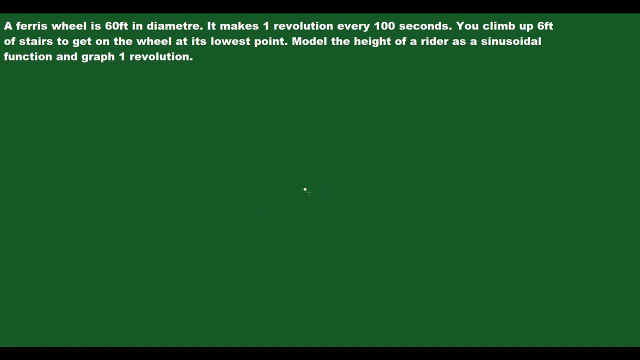 A ferris wheel is 60 feet in diameter. It makes one revolution every 100 seconds. You climb up six feet of stairs to get on the wheel at its lowest point. Model the height of a rider as a sinusoidal function and graph one revolution. Okay, so I like to start with a sketch of what's. 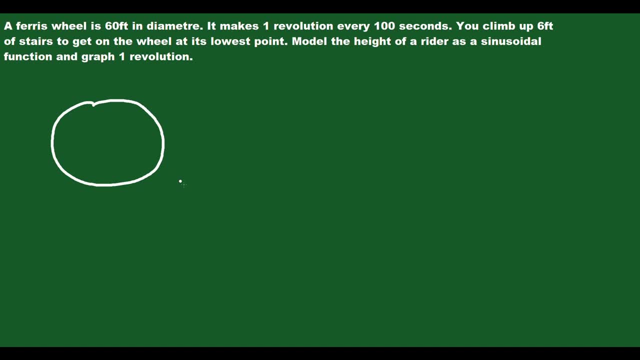 going on here, right? So you have a ferris wheel- looks something like that, right, And usually a ferris wheel, you know it has these sort of support legs like that and they're on the ground, and so here we'll draw the ground here like that, and we're told that you have to walk up six feet. 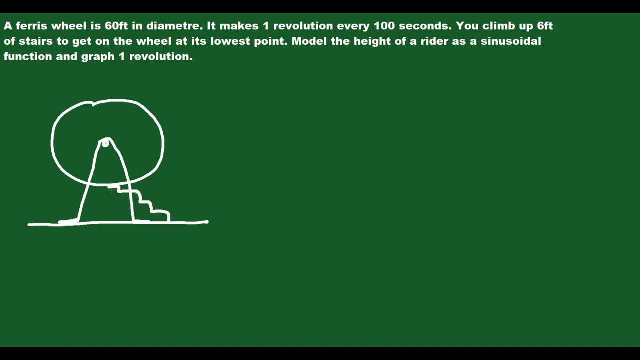 of stairs to enter the ride right. So you have this sort of step here and then you get on the ride here. Now the height of these stairs, they tell us, are six feet. Okay, we also know the diameter of the wheel is 60 feet. So from the very top of the wheel to the very bottom of the wheel. 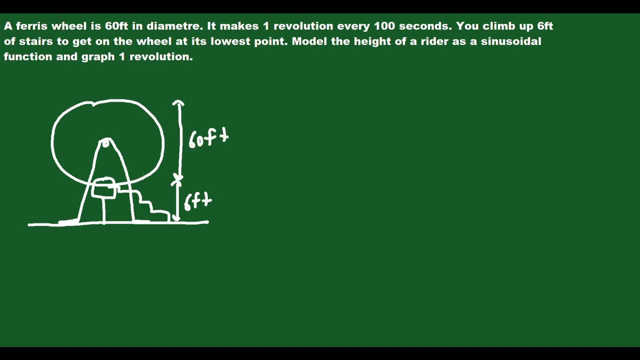 like this: that's 60 feet, right, That's the diameter. Obviously, this isn't a scale, but that's okay. We also know that it makes one revolution every 100 seconds, So we're going to keep that in mind, and now we're going to try to model the height of a person on the wheel, starting at the bottom, as 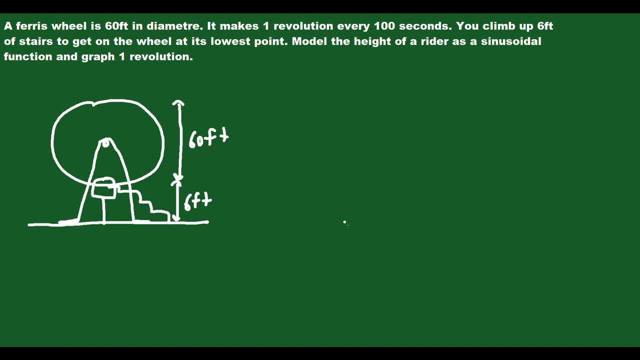 you go around using an equation. Now I like to make the graph first. They ask you to graph one revolution after, but I find it easier to make the graph and then make the equation, So let's go ahead. We'll make our axes like this: This will be t. this will be h at t. right, Your height at a. 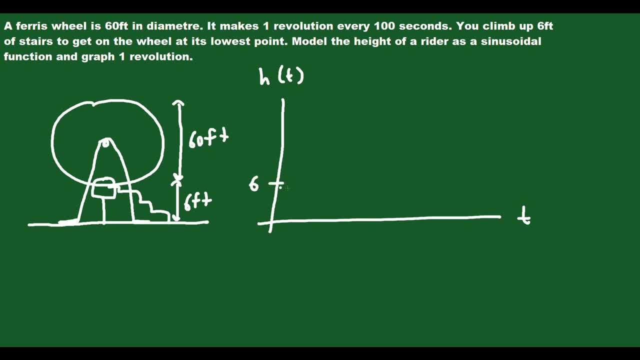 so when you enter the ride, you get on at a height of six, right. So you start off at a height of six and your maximum height is 60 feet above where you enter. Well, you're already six feet off the ground. so six plus 60 means you're 66 feet off the ground at the very top. So that's your maximum. 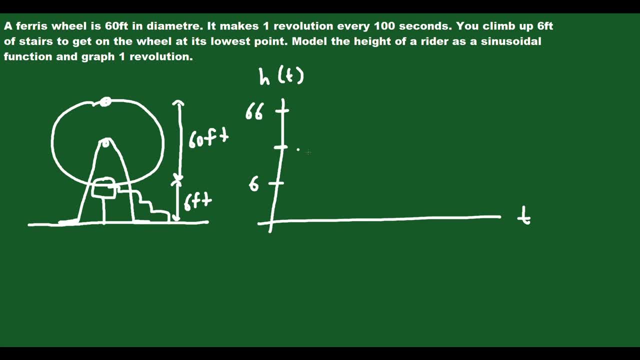 height. If you want to know where you're at in the middle right, The equation of your axis, which you should know, right, You should label It's going to be halfway between 6 and 66, of the circle, That distance is 30. So when you're in the middle, you're 36 feet off the ground. So 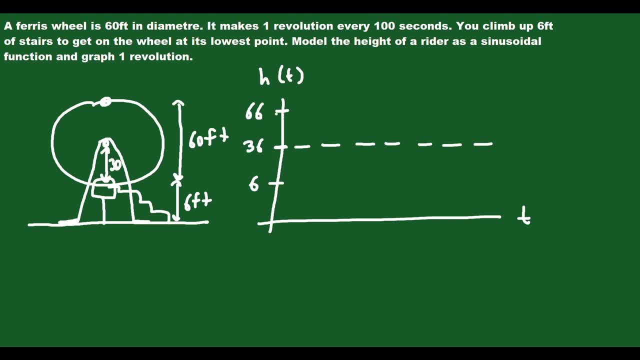 this is that 36.. And sure enough, 36 is halfway between 6 and 66, right, It's 30 more than 6 and 30 less than 66. So it is right in the middle. So it makes sense. What's also nice about this? 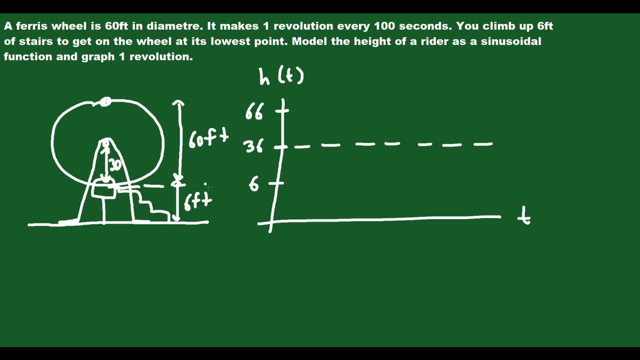 process is everything kind of lines up Like your minimum value lines up with your minimum value, the ground lines up with zero, the axle of the wheel lines up with the axis of the graph and then the maximum point lines up with the maximum point on the graph. Everything. 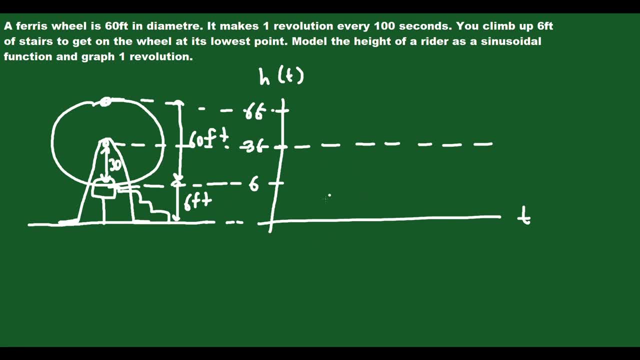 lines up nicely Now. with that in mind, we can go ahead and graph this So you start at a minimum value of 6 and then you start going around the circle and you start going up, And you keep going up and you get to the maximum value and you start coming back down And then you sort of come back. 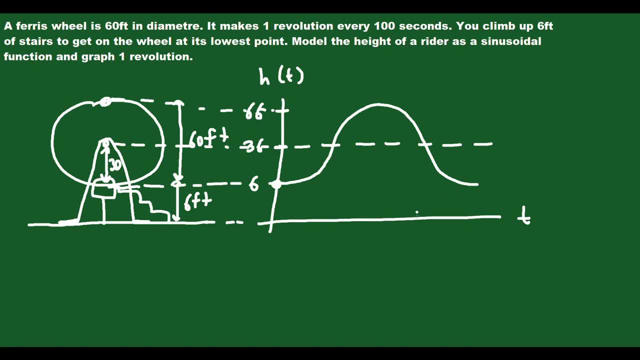 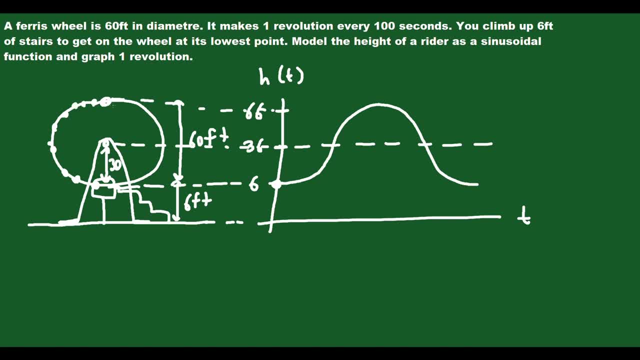 Then you get to the middle, Then you keep going up to the top and then you start slowing down as you get to the top, right, Like right here you're going up pretty fast, right, But over here you're kind of going up pretty slow, You're slowing down. You can see that in the graph right You start. 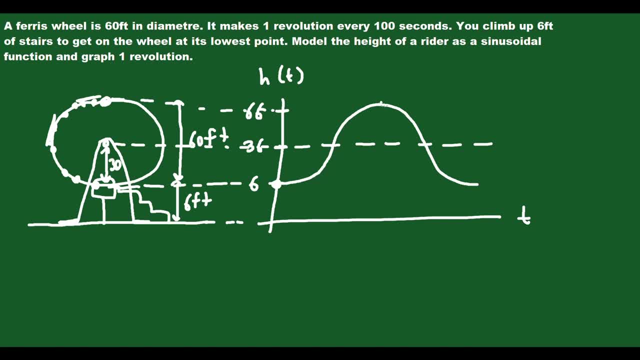 slow. then you get fast, right, It's going up very quickly and then it kind of slows down. Then it gets faster again and then it starts slowing down Again. you're not actually moving faster or slower, It's just that your height, right, Your change in height, is changing more quickly or more slowly. 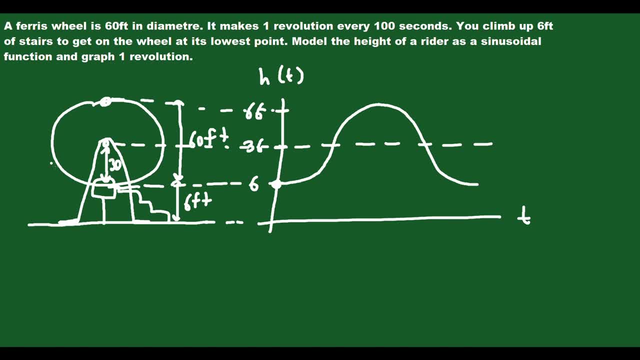 right, You're not going faster or slower, It's just the height is changing more slowly, Because for this section here you know, you're moving a lot horizontally but not much vertically right. And then in this section, here you know you're moving a lot vertically but not much. 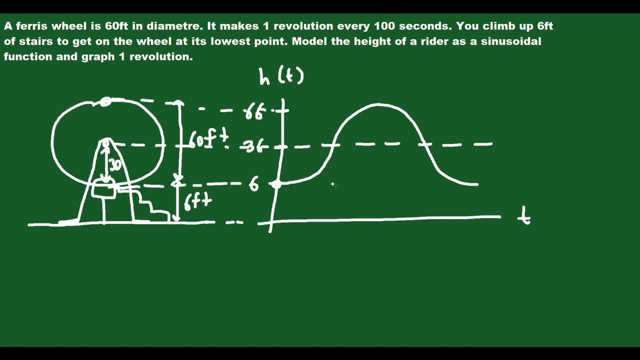 horizontally. This only measures the change in your vertical direction, right In your height. Okay, so now the last thing we have to label on this graph is the period. Well, we know you make one revolution every 100 seconds, So at this point you must be at 100 seconds, meaning that at your 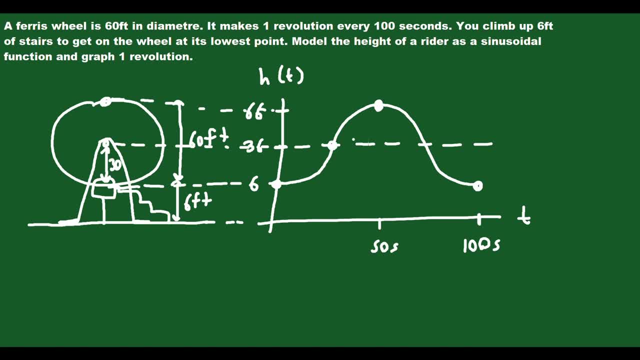 maximum, you're going to be at 50 seconds, Right, And when you're at your averages, right that 36 foot mark, you're going to be at 25 seconds and 75 seconds, right? I'm just dividing 100 into four sections here, right? So 0 to 25,, 25 to 50,. 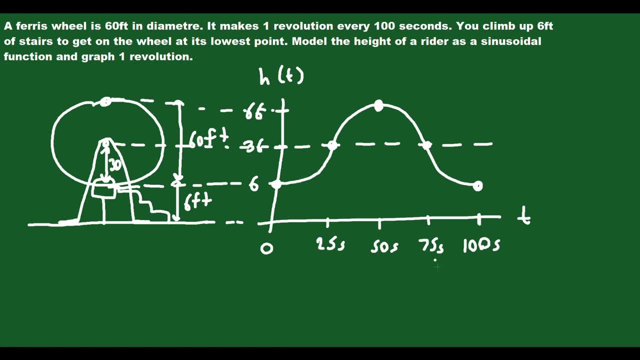 50 to 75,, 75 to 100.. Pretty self-explanatory, right? Okay, now we have to actually come up with the equation for this. So I'm going to say: h at t is equal to now when we write this out. 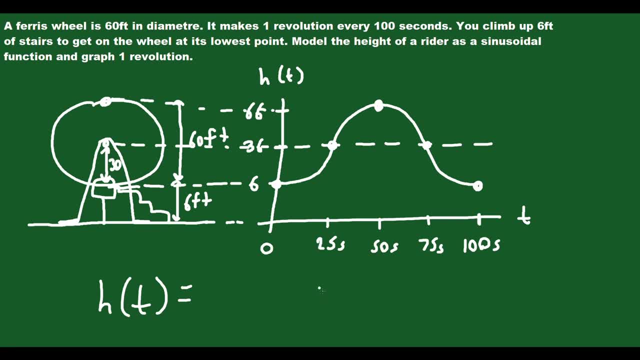 we have to make a decision. Do I want to use sine or do I want to use cosine for this function? Well, it kind of looks like an upside down cosine graph, right? Because remember, cosine just goes like that: It starts at the top, goes down, comes back up. So I think we 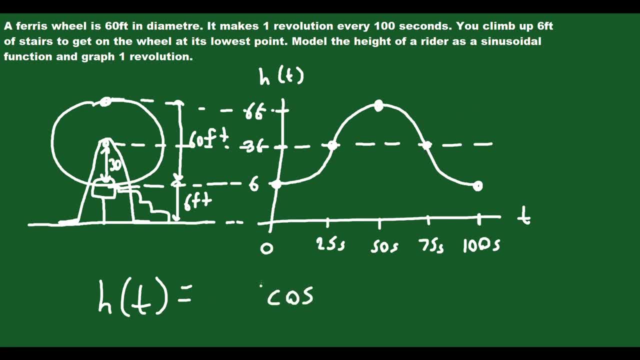 should use cos. So I'm going to use cos. What would my amplitude be? right, Because the amplitude is the thing that goes on the front. Well, the amplitude is the distance from the middle to the top, or the middle to the bottom. Well, that's just your radius in this case. right, It's the 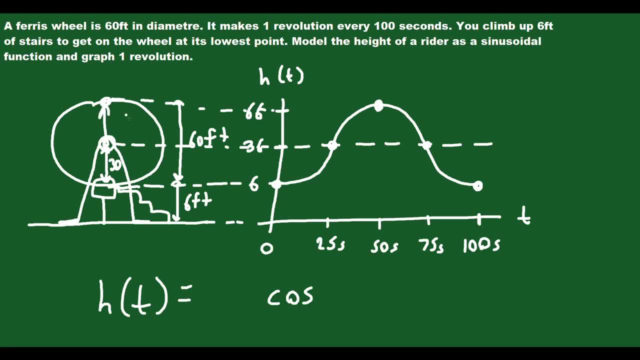 distance from your middle to the top or middle to the bottom of the circle right of the wheel. In this case, your radius is 30, right, We talked about that. Now, if you forgot, you can measure this distance right from 6 to 36, or 36 to 66.. Those are both. 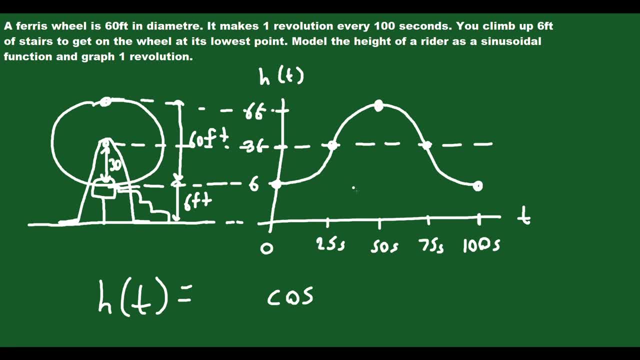 equal to 30.. So, of course, your amplitude for this one is just going to be 30.. So you put 30 on the front. And now remember what we said, that this is the upside down version of the cosine graph. So 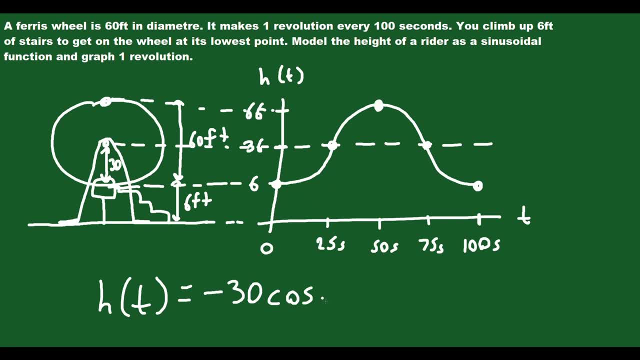 it's been vertically reflected, So we need to make that negative 30,. okay, Now, what else do we know? Well, we know that the axis right here is at a height of 36.. So I can say plus 36 on the end of. 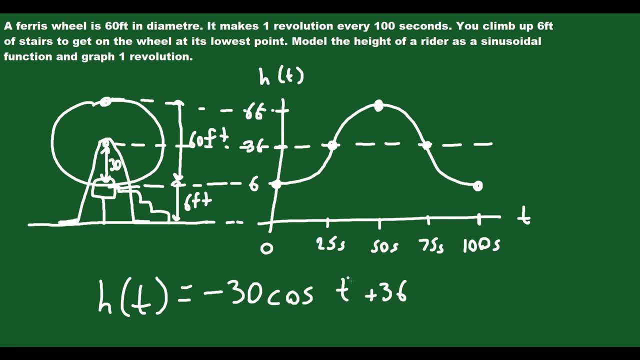 this equation right? I know I have t and that's not being shifted left or right because it's just an upside down cosine graph. right, There's no phase shift. We're not moving to the left or to the right. The only thing that I need to find is this k value here on front of the t to change the. 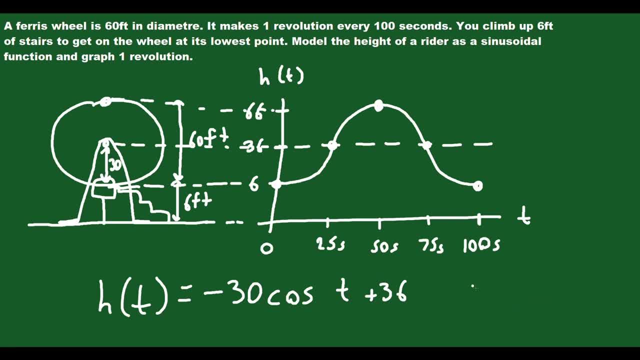 period, right? So I have to recall what's that relationship? Well, k is equal to 360 degrees divided by the period, right? Or you could say: the period is equal to 360 divided by k, right? Those two are interchangeable. So how do I find the k? 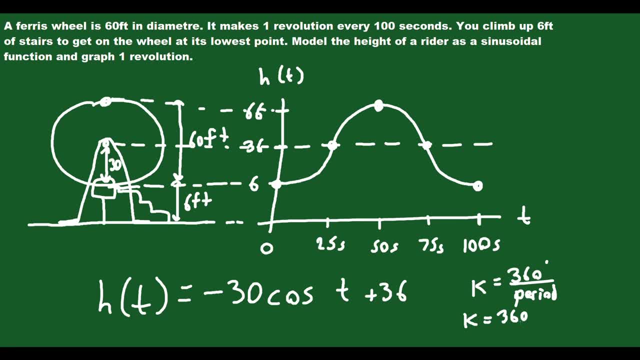 I plug in my period, which is 100 seconds. So 360 divided by 100, which is equal to 3.6.. So 3.6 is what I'm going to plug in right here, 3.6.. You can put that in a bracket if you want. So it's 3.6 t. 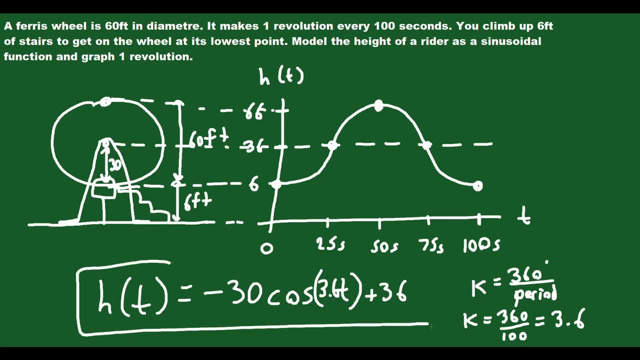 is what I've written there. This is the equation or the function that represents this scenario where you're going around the Ferris wheel. Now, let's say they asked you some follow-up questions, right? I mean, what if they asked you? 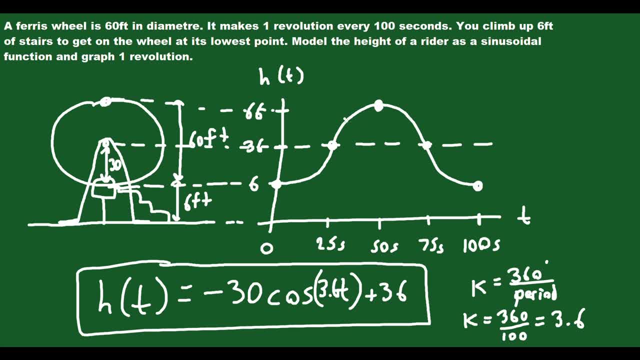 how high are you At a particular time? right, Like if they said: at 25 seconds, what's your height? Well, you can look at the graph and see: okay, 25 seconds, you go up. you know you're at 36 feet, But they could ask: 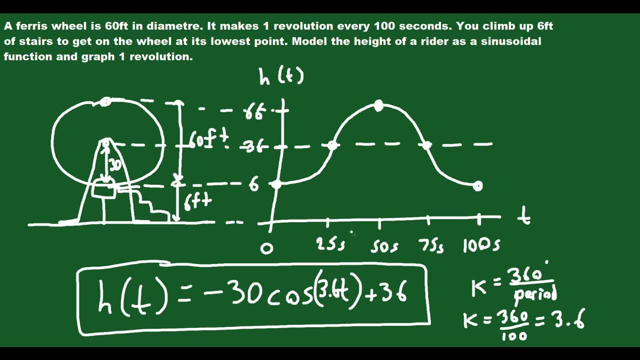 you. you know something more specific. They could say, at 27 seconds: how high are you? Well, you would go and you'd realize: okay, I'm a little bit above 36 feet, right, But how high is that? 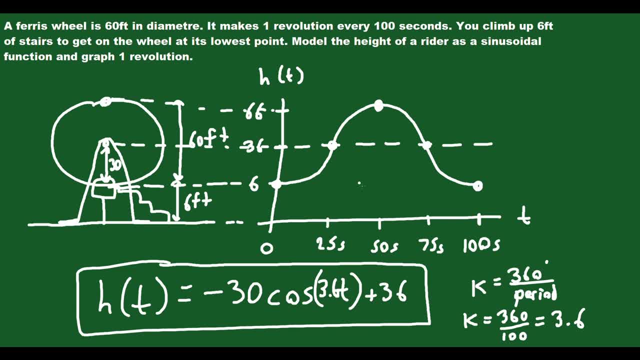 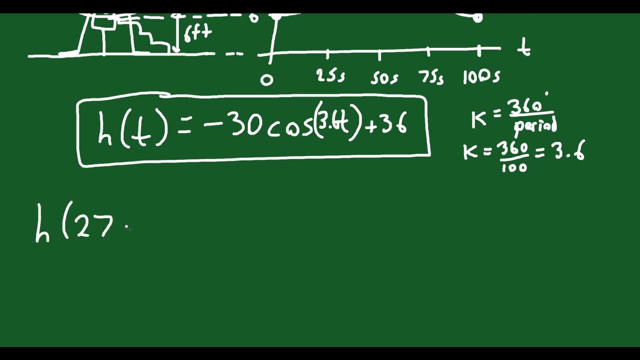 exactly. Well, all you would have to do is plug in 27 into your formula right, Find h of 27 and calculate it. We can actually do that right. If I want to find the height at 27 seconds, I'm going to. 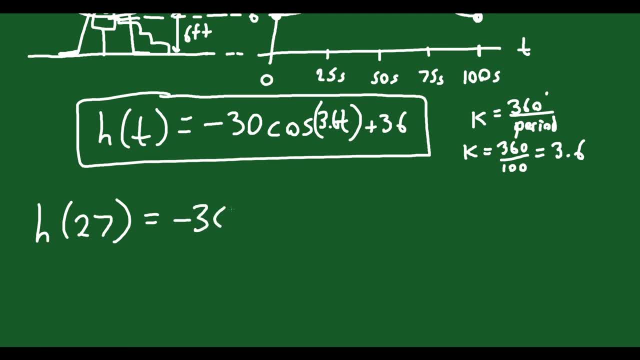 plug in 27 for t, So you'd have minus 30 times cos of 3.6 times 27 plus 36.. And then you would just go ahead and you would calculate this, And when you do that you get an answer of 39.76 feet. 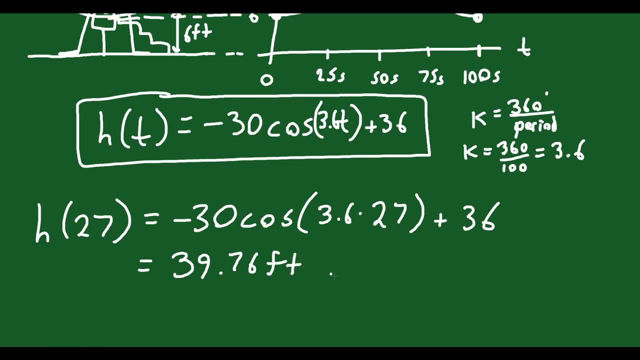 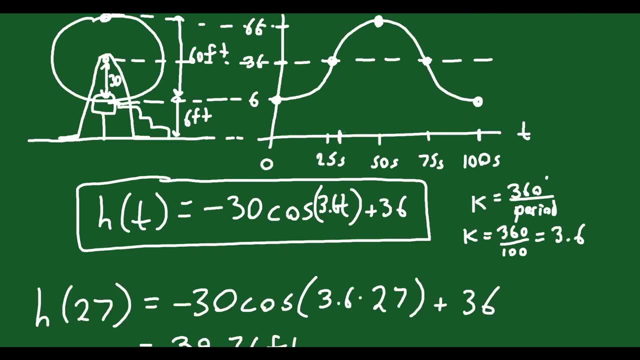 approximately right. If you round your answer So 27 seconds, you're at 39 feet And that makes sense with the graph right. 27 seconds would be about here, a little bit after 25.. And that would put you at a height of 27.7.. So you'd have minus 30 times cos of 3.6 times 27 plus 36.. And then you 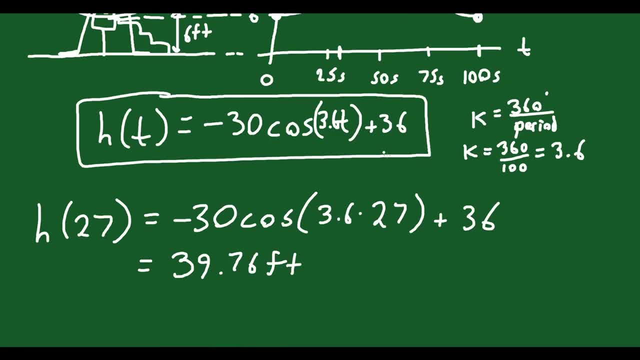 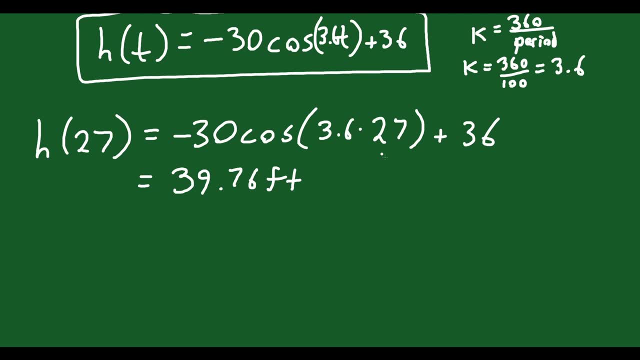 a little bit bigger than 36, right, Like the one we found, 39.76.. So that makes sense. Now they could also ask you a question like: at what times are you at a height of 40 feet? right, So you look at. 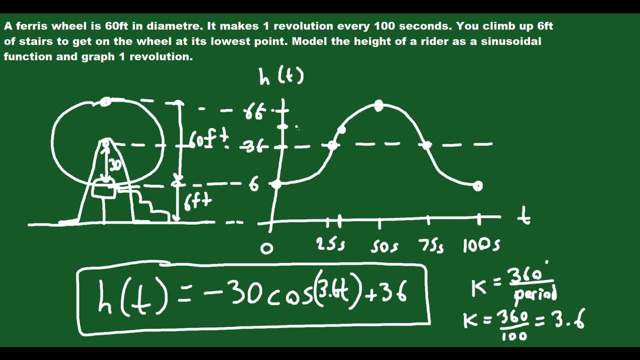 the graph here and you say: okay, well, 40 feet is about here, right? And then you can look and you can say: okay, where's you know this point and this point, because that's also at that same. 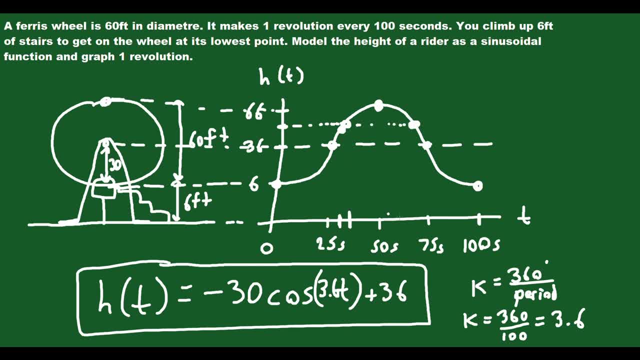 height right. And then you look down and you see: okay, here and here, what are those times. How do you find that? Well, to find those, all you have to do is find the height of 30 feet, And then you. 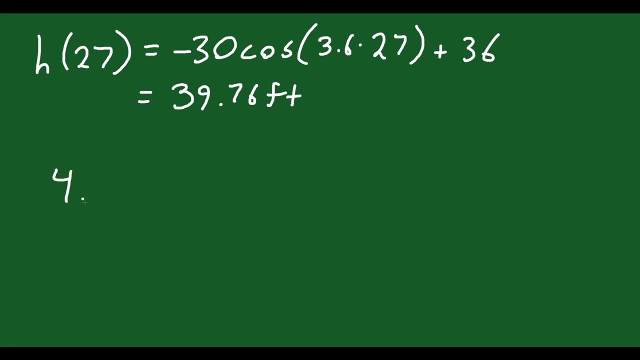 plug in 40 for your h and solve for t, right. So 40 equals negative 30 cos 3.6 t plus 36.. Now let's try to solve for t. You move 36 to the other side. So 40 minus 36 is 4, right. And then? 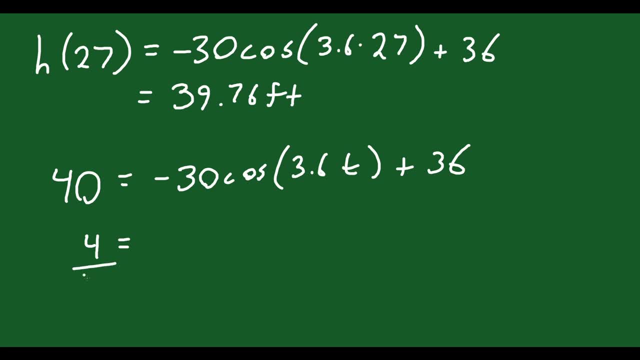 you want to divide by 30, right, Divide both sides by 30. So you'll have negative 4 over 30 is equal to cos of 3.6 t, And then I need to get rid of cos, So you're. 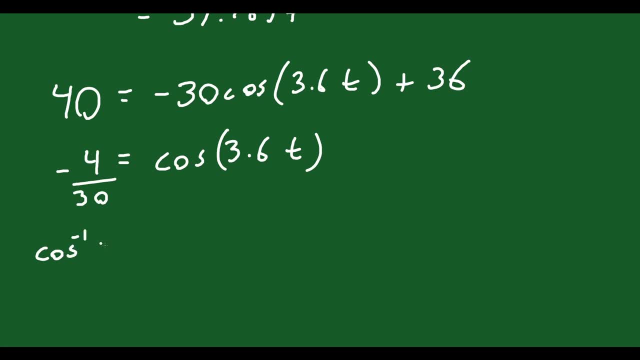 going to take the cos inverse of both sides. Cos inverse of 4 over 30 equals 3.6 t. If you do cos inverse of 4 over 30, you get 97.66 approximately. That's equal to 3.6 t. Divide both sides by 3.6. 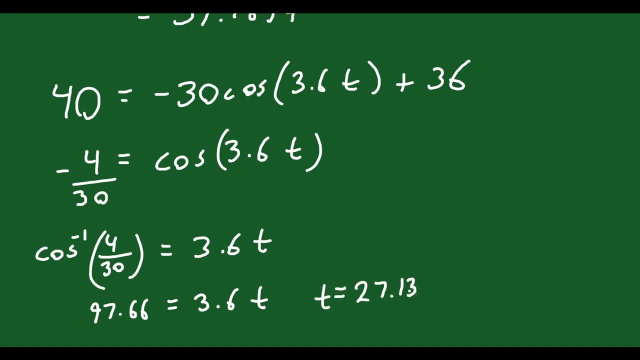 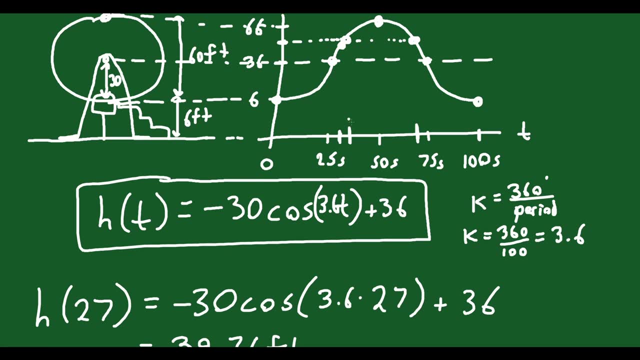 and you're going to get t is equal to 27.13 seconds. Now 27.13,. if you look at the graph up here, it makes sense right. This time here, 27.13.. That makes sense, right, It's right. after 25,. just a little bit to the right. 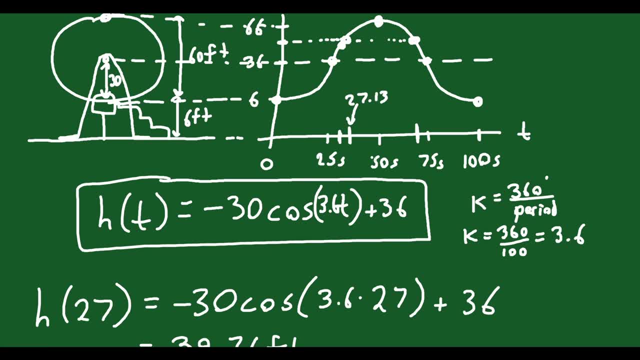 Kind of similar to the question we just had right, Similar numbers anyway, But that's just one time right. That gives you the time when you're at this height right here But you're at the same height over here. How can I find that time? Well, thankfully, these functions are. 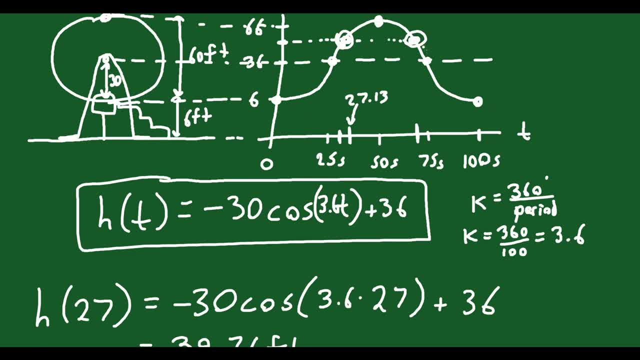 symmetrical and they're cyclical right. They repeat over and over again, So we can find out what this one is, if we know what this one is right, Because this is the same distance from here as this time will be from the end, So we can actually determine that well, this distance is. 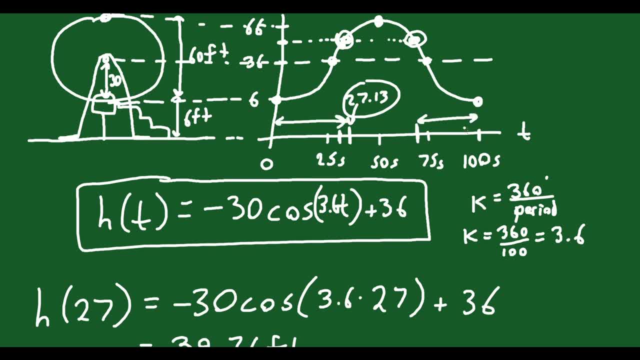 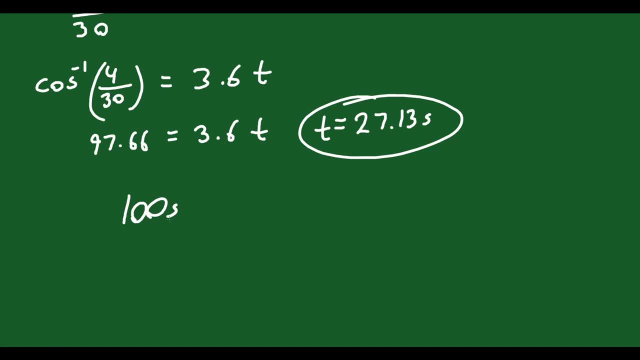 27.13.. This distance here is also 27.13.. So I can subtract that from 100 seconds. So I can say 100 seconds minus 27.13 seconds and that's going to give me 72.87 seconds. So that's the other time. 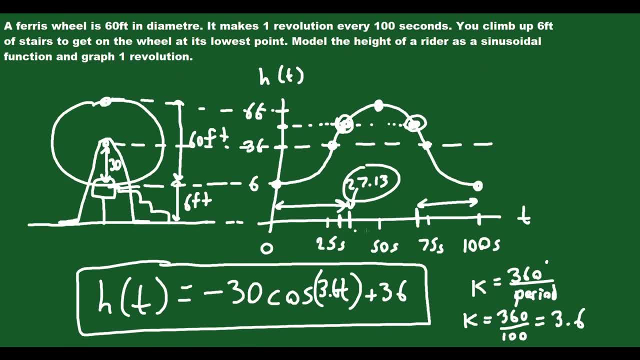 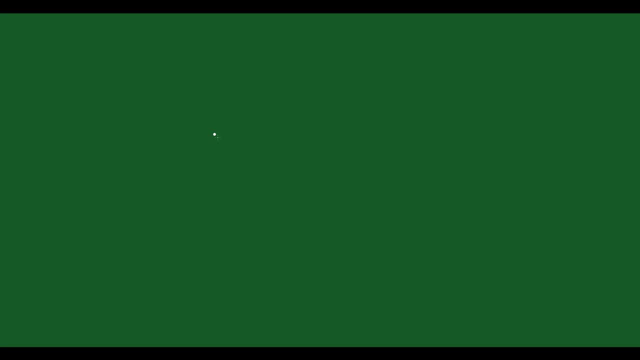 when we're at this height. And if you look at the graph, it makes sense right. Right here is 72.87.. Because, look, it's right before 75 seconds. So it makes sense. right, The answer here makes sense. Okay, let's do another example. Let's say you're told that the hottest 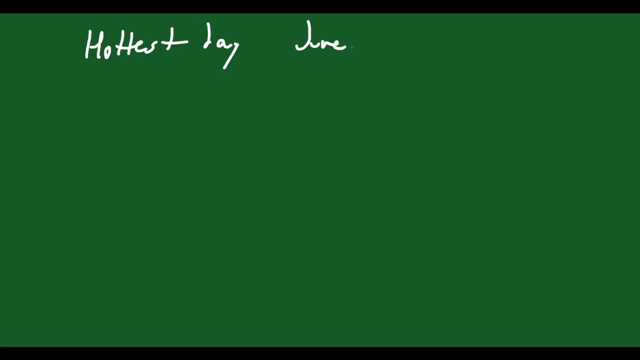 day of the year is June 7th, And on June 7th it's 29 degrees Celsius. And let's say, we're told that the coldest day of the year is. well, we don't know what it is actually. We're not told that. 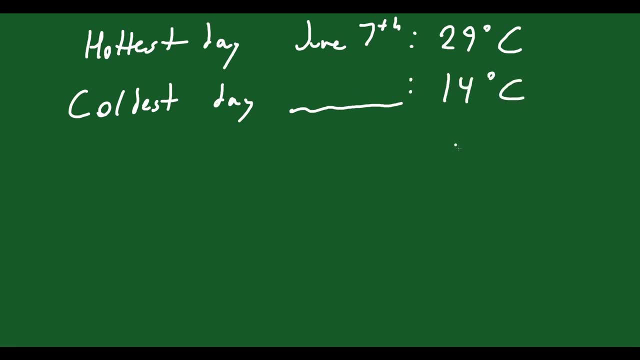 But we know that it's 14 degrees Celsius on that day. All right, and this is on average at a particular time, Using a trig function right or a sinusoidal function. model the temperature using 365 days. Okay, so we got to model the average temperature every day for a year. 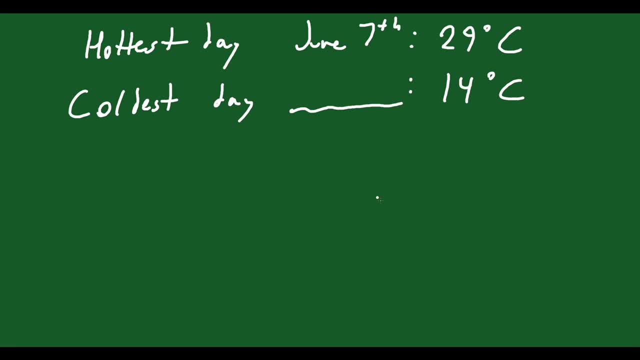 And then they're going to ask you how many days after June 7th is the first spring day when the temperature reaches 20 degrees Celsius. So that's an additional point. We'll get to that later, So for now, let's just try to model this right So you have a function We're going to set. 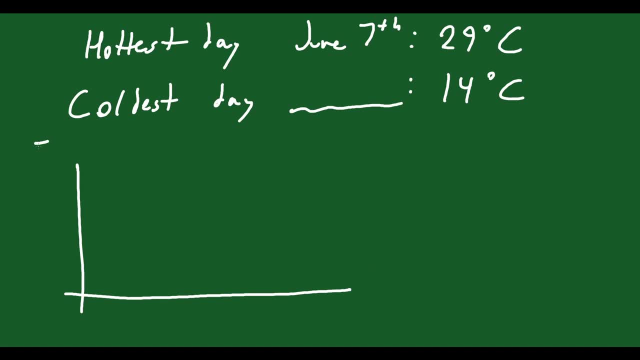 up our axes like this: Over here we'll have the temperature in terms of the day And on this axis I'll have D for days, But that's going to be days after June 7th. We're going to start on June 7th at the maximum day, up here at 29 degrees Celsius, Okay, and then down here. 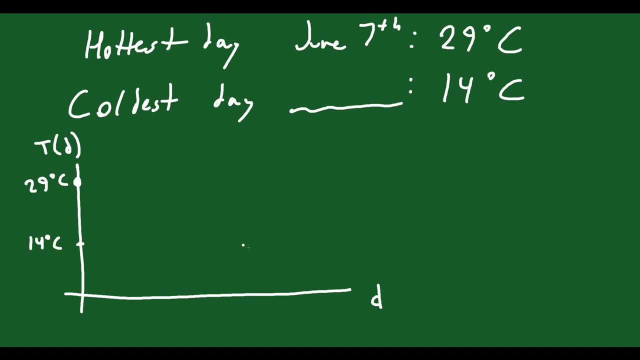 you'll have 14. Degrees Celsius- that's the coldest day, right? So we start at the top and this is just going to follow that same sinusoidal pattern, right? It repeats, So it's like a cycle. It goes up and 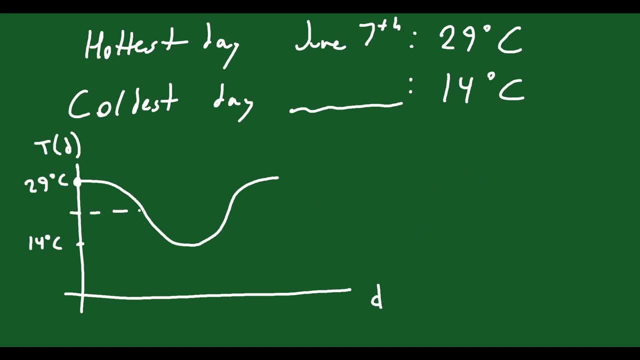 down and up and down, up and down keeps repeating itself. Now, there's lots of things here we can find right. We can find the axis or the midline. right It's 29 plus 14 divided by 2,, right It's. 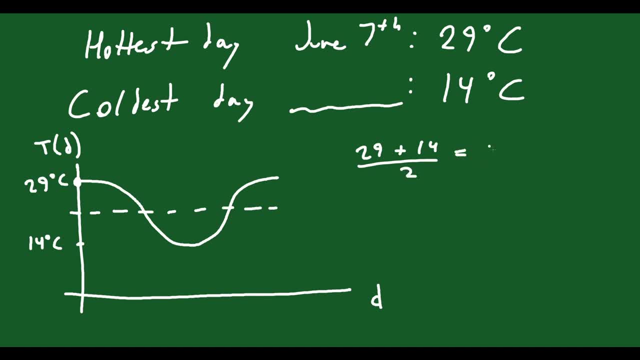 the average between those. If you do 29 plus 14 divided by 2,, that's equal to 43 over 2, or 21.5.. So 21.5 is going to be the average. We can label this here, day 0,, as being June 7th, And then when? 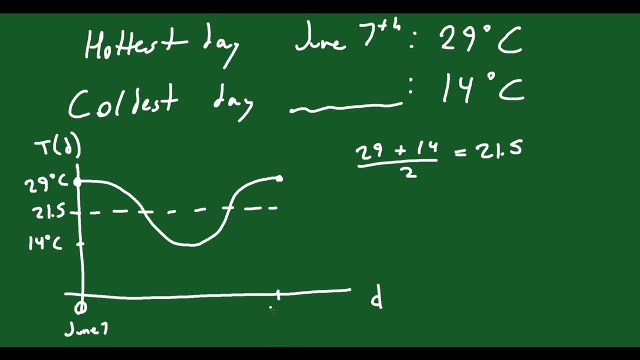 we get to that point again up here, that'll be day 365, which we know is also June 6th. right, It'll be the day before, because then it just repeats the entire cycle over and over and over. And so now we can figure out what our equation looks like. right, We can say: T add D is equal to. 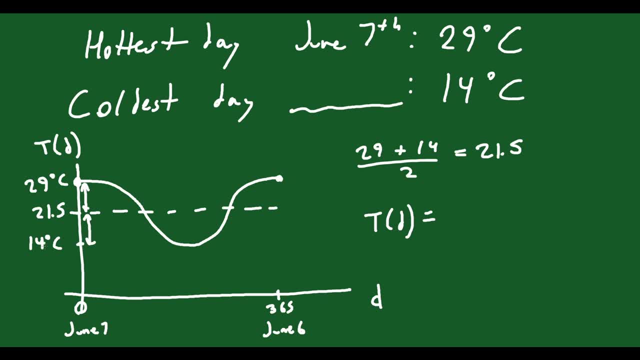 right. The amplitude is this distance or this distance. Distance from 14 to 21.5 is 7.5, right. From 21.5 to 29 is also 7.5, right. So the amplitude is 7.5,. okay, Now it's a. 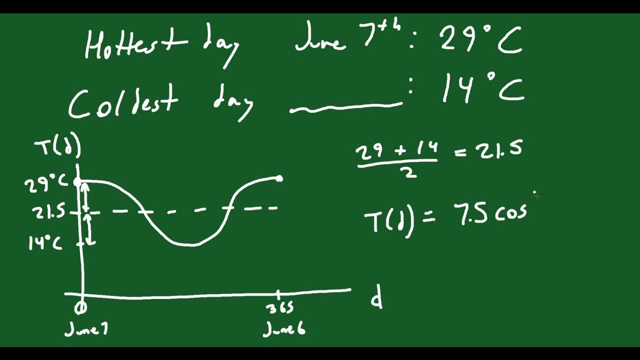 function. You can see that pretty clearly. So we'll put cos. I want to put some k value in front of D, but then I'll put 21.5 because that's the equation of the axis. right, That's your average. 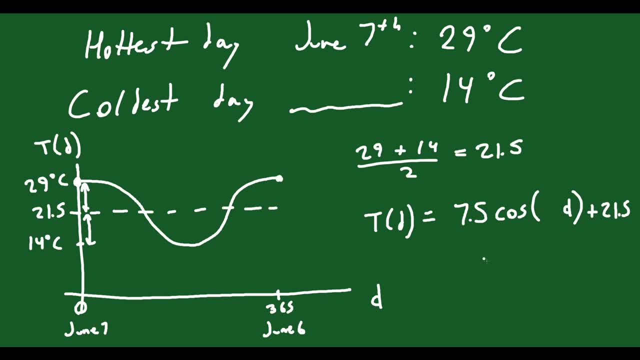 here, It's your midline. So what value for k can I put? Well, k, as we know, is 360 divided by the period. Well, the period's 365, right? So that actually reduces to 72 over 73. So I'll put that number in here: 72 over 73. That simply converts. 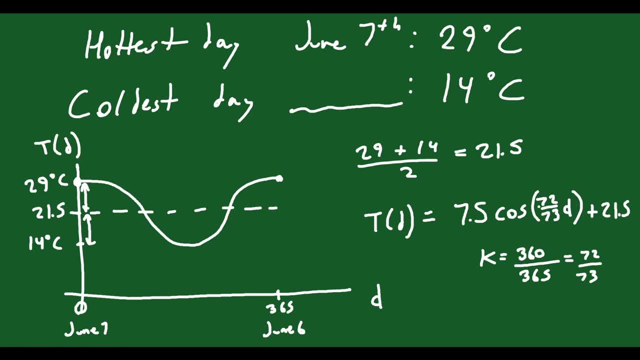 whatever number of days we put in here into a degree that the function cos can understand and interpret. okay, So that's the function. So that's part of the question already done. The other part of the question- I'll read this again- is: how many days after June 7th is the first spring day when temperatures 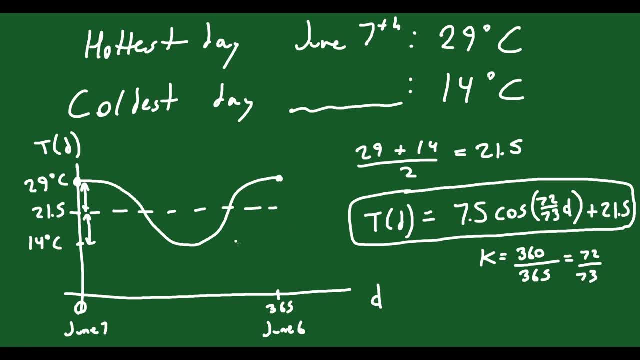 reach 20 degrees Celsius And they say first spring day because you obviously reach 20 degrees Celsius here, but at that point it's still getting colder, right, And as it gets colder you get to the winter. Now, as you come out of the winter, you're in spring. you get to 20 degrees. 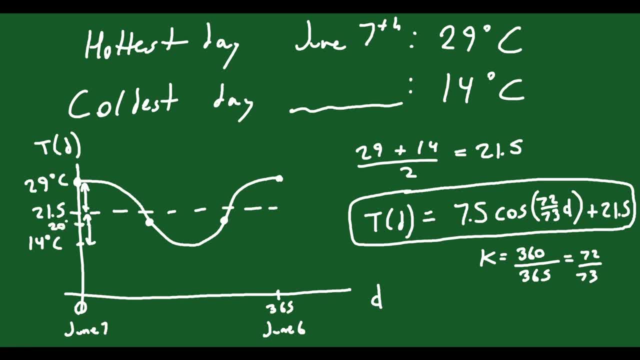 Celsius. again, right, I'll say this is 20 degrees Celsius, right? So you reach 20 degrees Celsius twice, while the temperature is dropping into the winter and while it's recovering into the spring and into the summer, right? So I don't want to find this time. I want to find this time here. 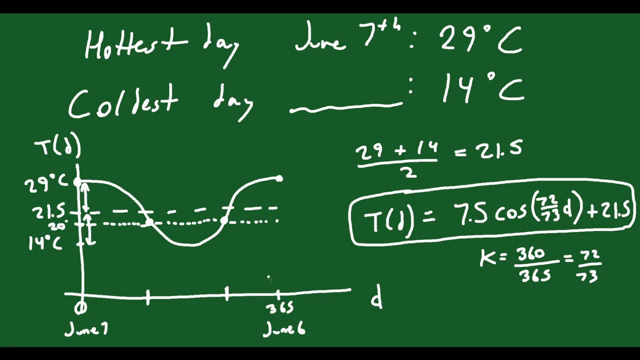 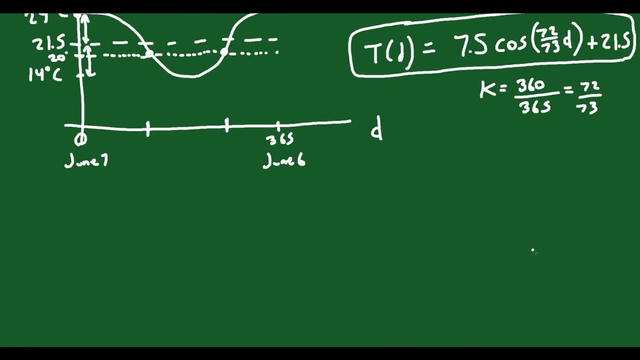 How many days is this after June 7th, right? Well, how can we find that We set the temperature to 20 and we solve for d? So let's go ahead and do that We'll have. 20 is equal to 7.5 cos 72,. 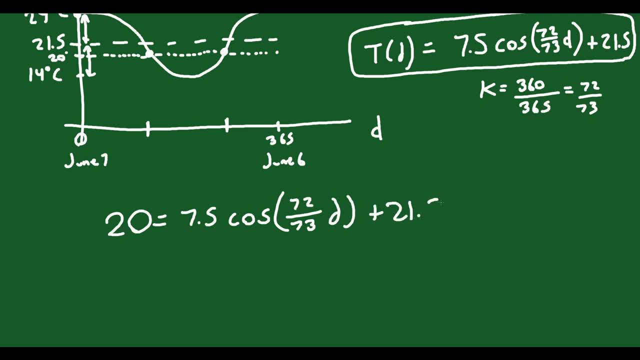 over 73d plus 21.5.. Okay, let's solve for d. I'm going to move the 21.5 to the left. 20 minus 21.5 is negative 1.5. Divide both sides by 7.5. So divide by 7.5. That's equal to cos of 72 over. 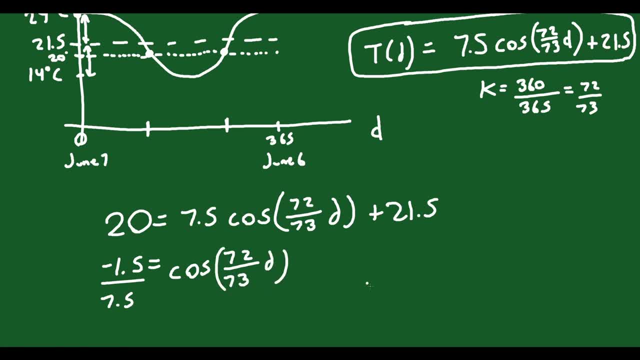 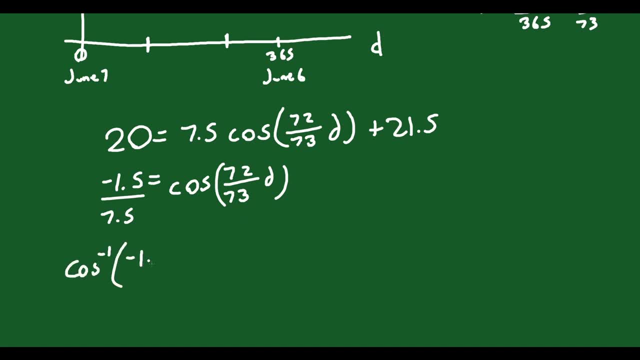 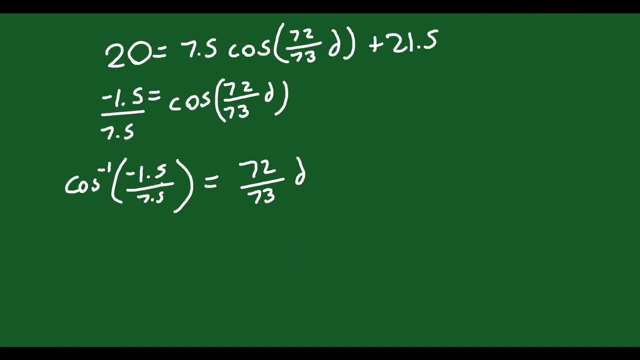 73d, just like that. I can now take the cos inverse of both sides. right Cos inverse of negative 1.5 over 7.5. Inverse on the right: it's just going to cancel. I'll get 72 over 73d When you cos inverse this.